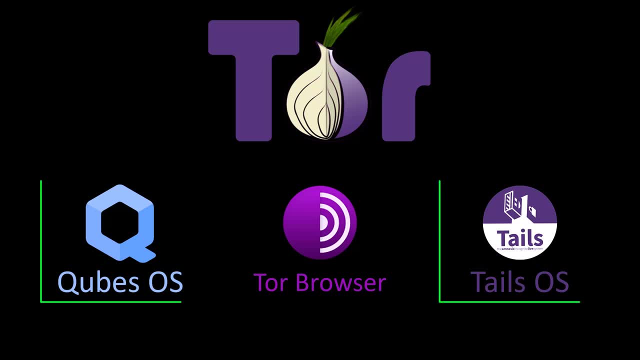 So, in fact, we will be using the Tor Browser in other methods that we consider safer in the continuation of the course. Since operating systems that we will use the Tor Browser for in the methods we consider safe are fully configured for privacy, they will provide a much more secure environment than any other operating system. 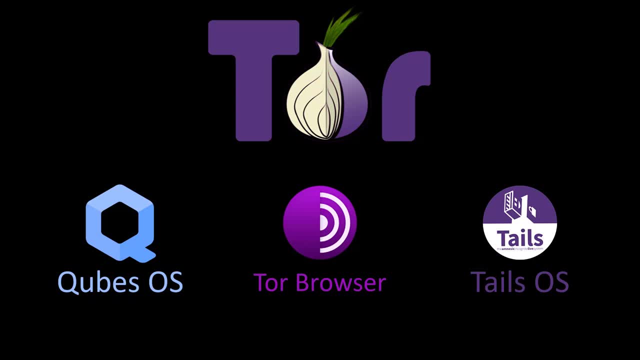 So actually using the Tor Browser on Android, Windows, macOS or a standard Linux distribution is not a completely inefficient way, But it is not the best way for security and privacy. The vulnerabilities that may occur in operating system or software on the operating system may cause the anonymity and privacy features. 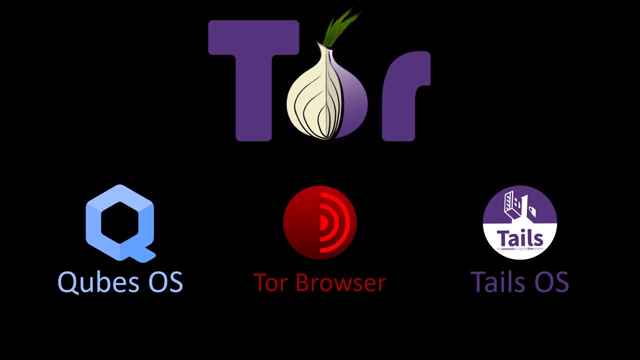 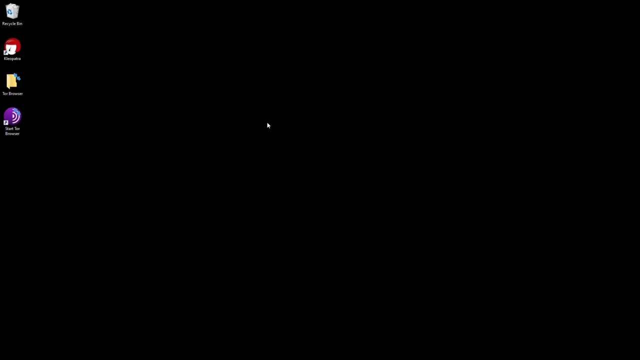 provided by the Tor Browser to become meaningless. In short, using the Tor Browser on standard operating system is practical, but alone is insufficient for security. Without further ado, let's continue to explanation by talking about the use of the Tor Browser and its various settings. 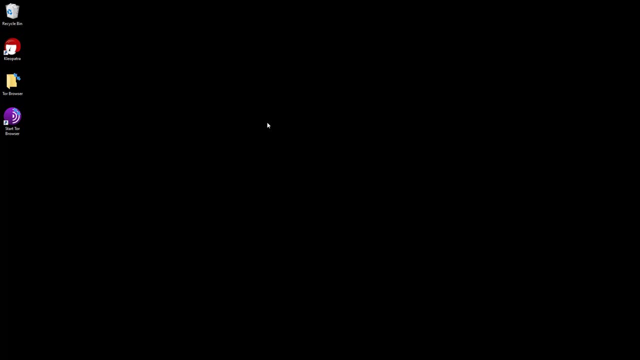 Although the installation and verification process differ slightly for different operating system, the use of the Tor Browser after it is installed is very similar for all system. In other words, all system user can easily follow the instruction here. I will perform the lectures on Windows operating system for now. 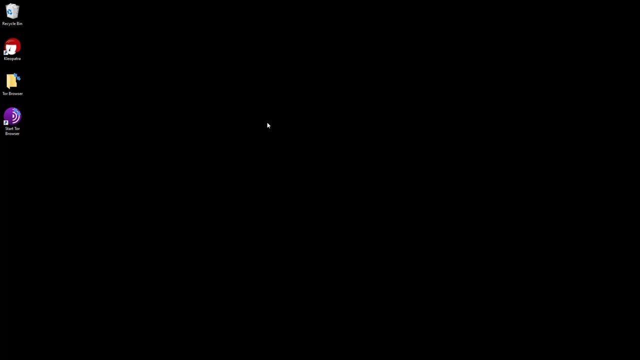 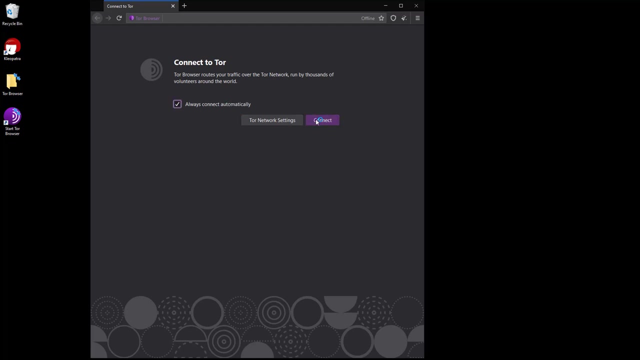 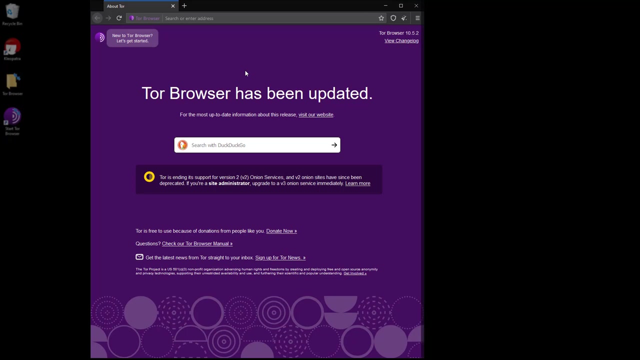 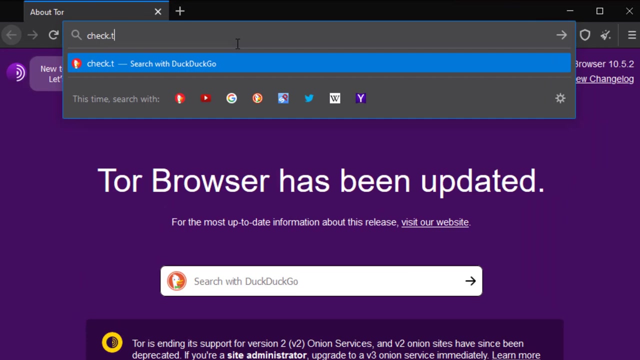 You can follow it on any operating system you want. I double click on the application to open the Tor Browser. As you can see, a simple browser interface doesn't look much different from the standard Firefox browser. welcomed us. Now let's check our connection by going to checktorprojectorg. 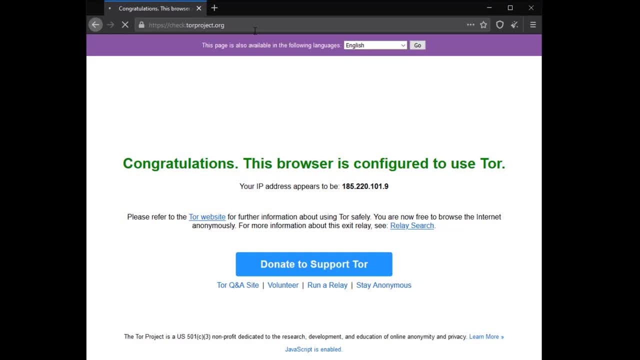 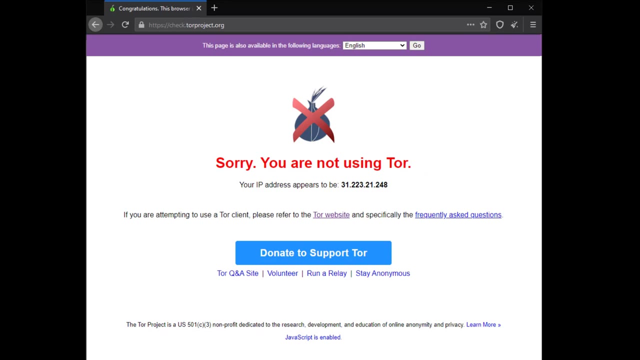 to test whether we are properly connected to Tor Network. On the page that opens, we can confirm that our connection is routed through the Tor Network, as it should At this point. if you haven't encountered this confirmation statement, you may have an internet connection. 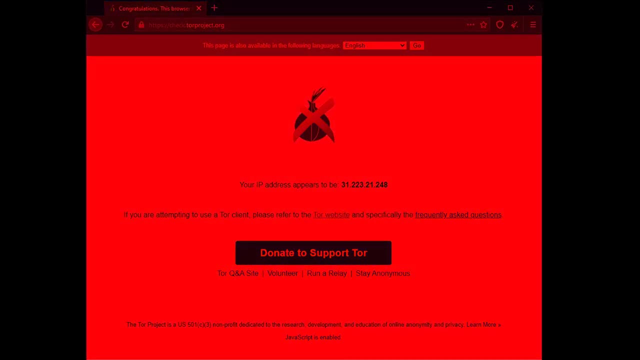 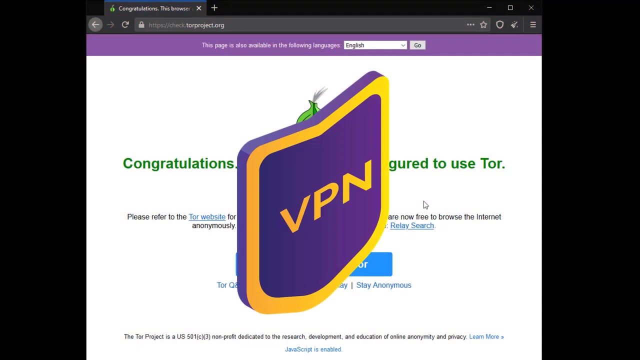 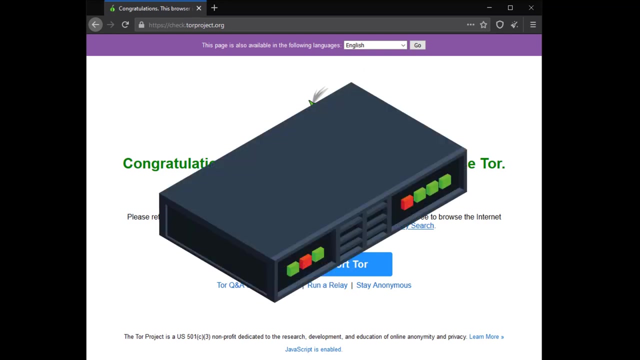 where the Tor Network is blocked. In such cases, you can choose to use the Tor Bridge Connection or VPN to bypass the block. We will talk about VPN usage in the following lectures. For now, let's continue with explanation by talking about the Tor Bridge Connections.